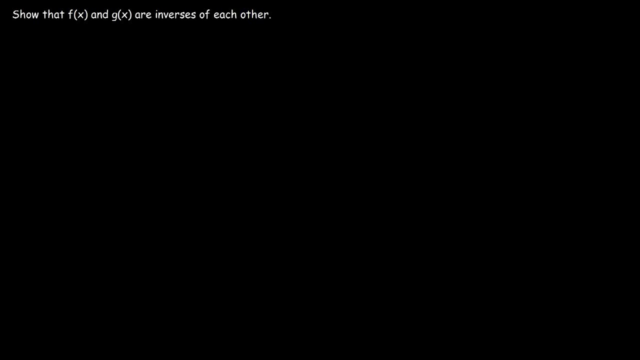 In this video we're going to talk about how to show that two functions, f of x and g of x, are inverses of each other. So let's say that f of x is equal to x squared plus 5, and g of x is the square root of x minus 5.. Are the two functions inverses of each other? 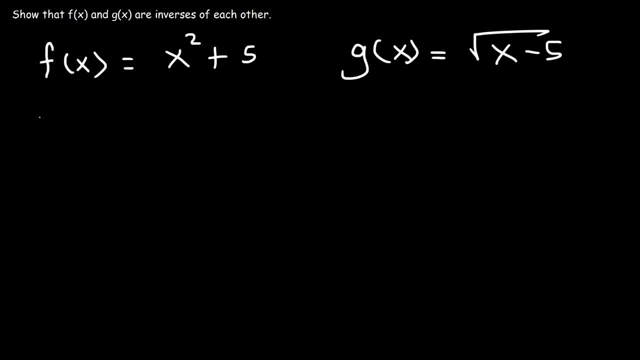 Well, let's see if they are. So what we need to do is show that the composition of the two functions f of g of x is equal to x and also, in the reverse order, g of f of x is also equal to x. If that's true, then the two functions are: 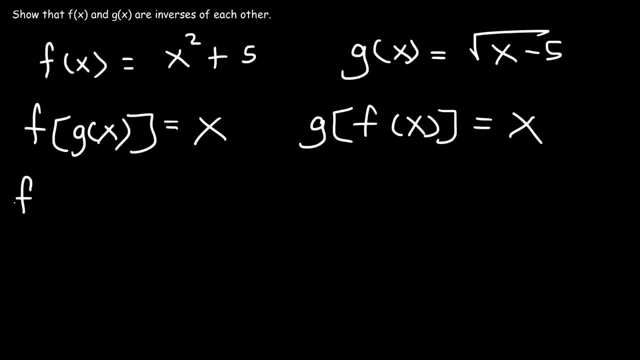 inverses of each other. So first let's determine f of g of x. So g is on the inside of f. So we're going to take this stuff and and insert it into f. So I'm going to replace x with the square root of x minus 5.. 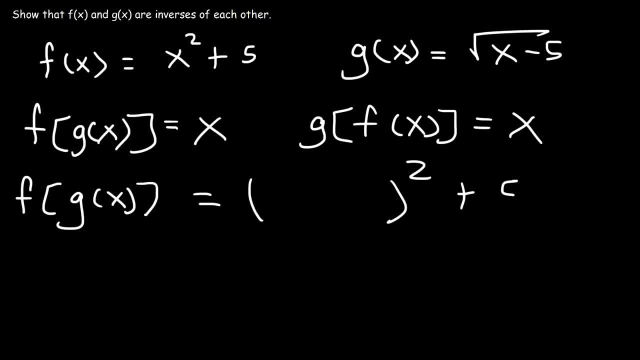 So normally this would be x squared plus 5.. That's the outside function f. The inside function g, I'm going to put it inside of f, So I'm going to replace x with the square root of x minus 5.. The square of the square root, these cancel, giving me what's inside. 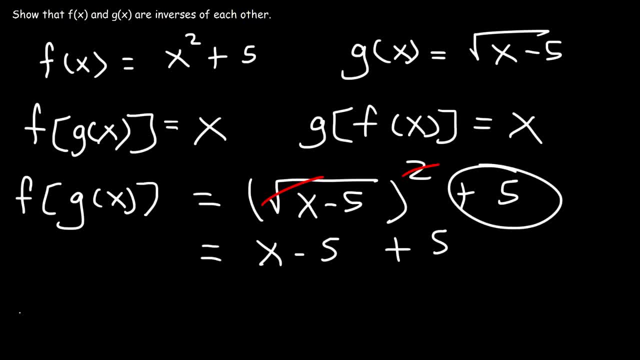 Which is x minus 5.. And then, if you add that to plus 5, negative 5 plus 5 is 0, leaving behind x. So f of g of x is equal to x. Now what about g of f of x? 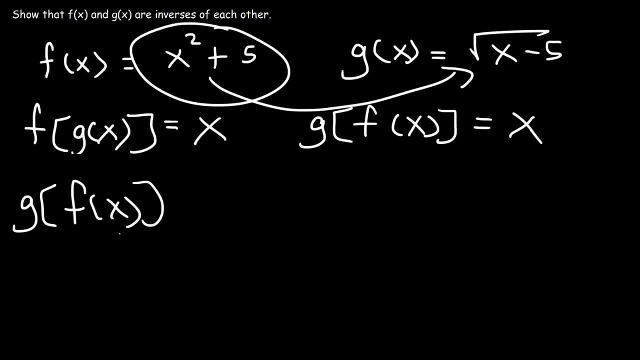 So I'm going to take f and insert it into g. So let's start with g. It's the square root of x minus 5.. So here's where x would be, And I'm going to take this and replace it or substitute it for x. 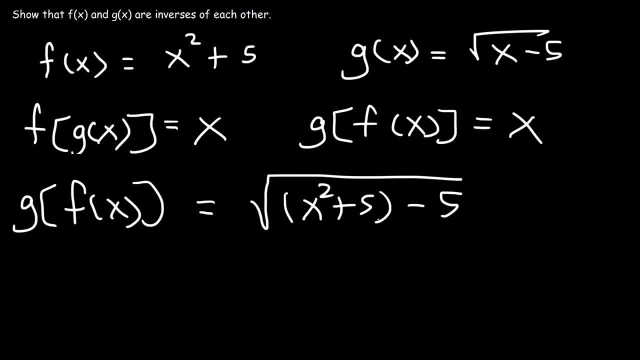 So that's x squared plus 5.. Now 5 minus 5 is 0.. So that leaves the square root of x squared, And the square root of x squared is x. So therefore these two functions are inverses of each other. 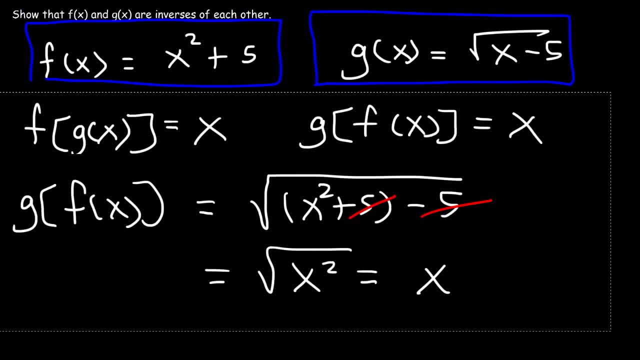 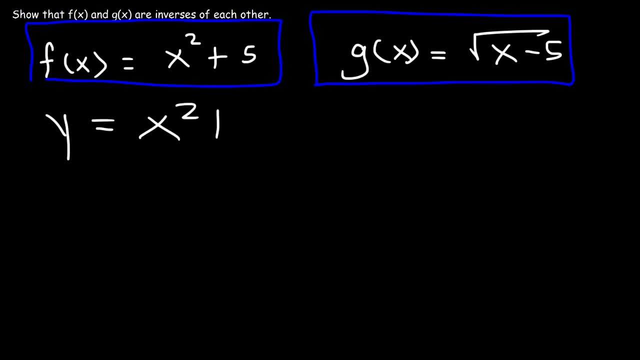 Another way you can confirm the answer Is by finding the inverse function of f. F of x and y are the same thing. So to find the inverse function, replace x with y, Next solve for y. So I'm going to subtract both sides by 5.. 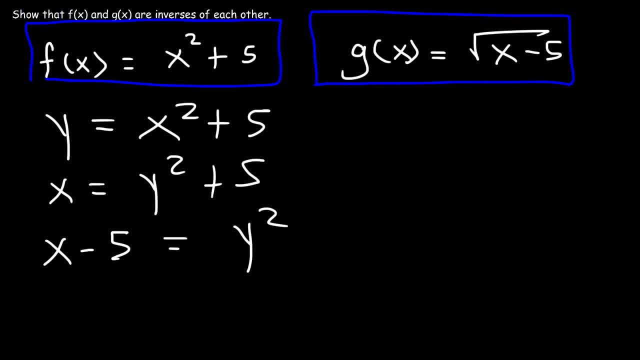 So x minus 5 is equal to the square root of y. I mean y squared. Now you need to take the square root of both sides. So the square root of x minus 5 is equal to y. So therefore we can say that x minus 5 is equal to y. 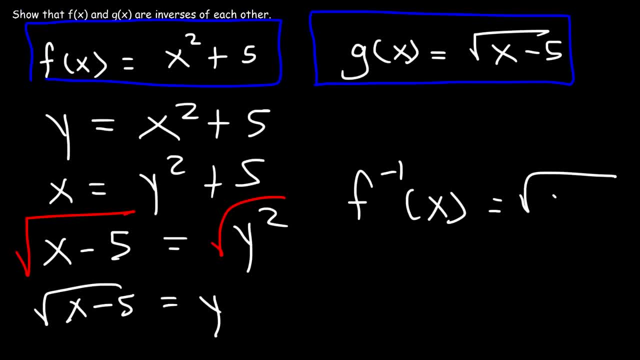 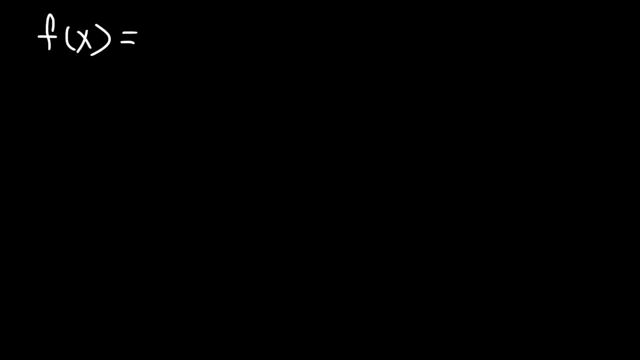 Now let's say that the inverse function of f is the square root of x minus 5. Which is the same as g of x. So f of x and g of x are indeed inverses of each other, Number 2.. Let's say that f of x is equal to 3x plus 8.. 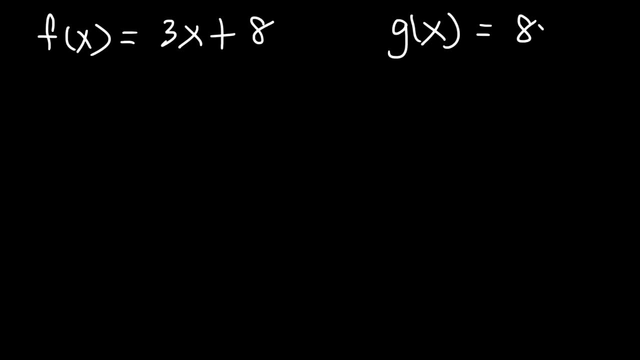 And that g of x is equal to 8x squared minus 3.. Are these two functions inverses of each other? No Well, first let's determine f of g of x. So let's start with the outside function f. So it's 3x plus 8.. 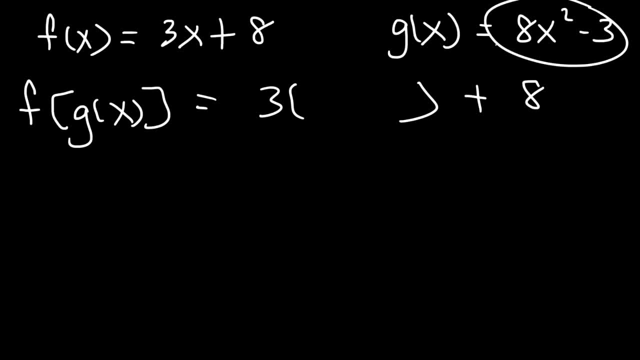 But then let's replace x or substitute it with 8x squared minus 3.. Now let's distribute the 3.. 3 times 8x squared is 24x squared, And then 3 times negative 3 is negative 9.. 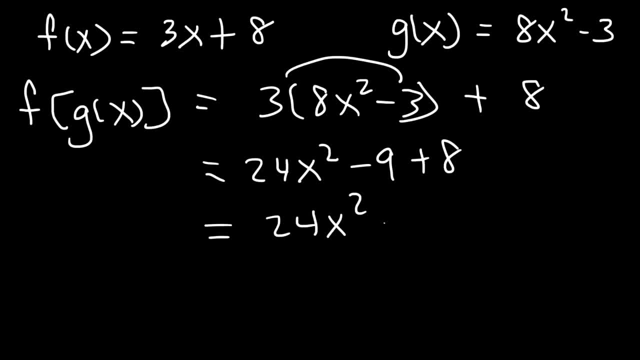 Negative. 9 plus 8 is negative 1. And we can't simplify this any further. So notice that this does not equal to x. So since f of g of x does not equal x, then g is not the inverse of f. 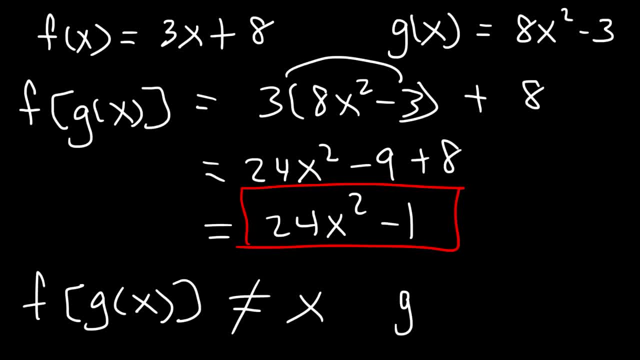 And f is not the inverse of g. So we can say g of x is equal to 3x squared minus 3x squared, minus 3x squared, minus 3x squared, And then f of x is not the inverse function of f. 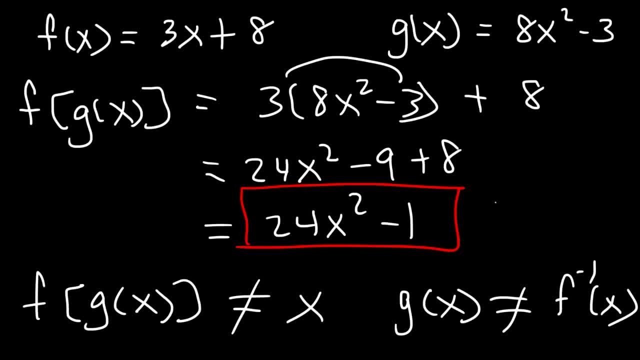 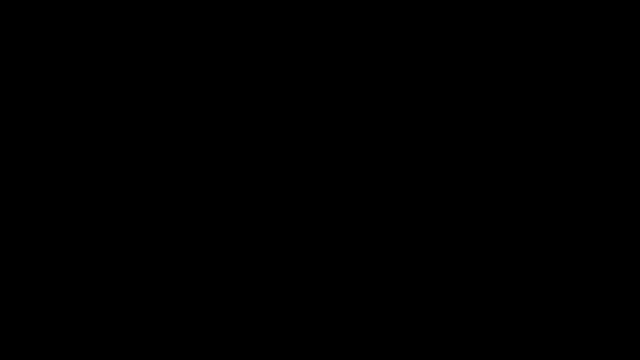 And we could also say that- Let me make some space- We can say that f of x is not the inverse function of g of x, Because this is not true. Now let's move on to another example. So let's say that f of x is equal to a squared minus 9.. 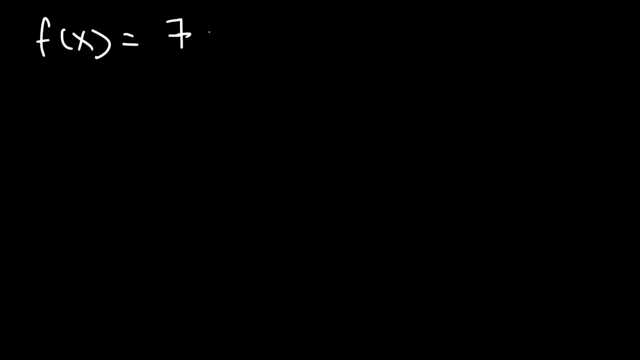 And that g of x is equal to 3x squared minus 3x squared minus 3x squared minus 3x squared is 7x plus 5.. And that g of x is x minus 5 divided by 7.. Are these two functions? 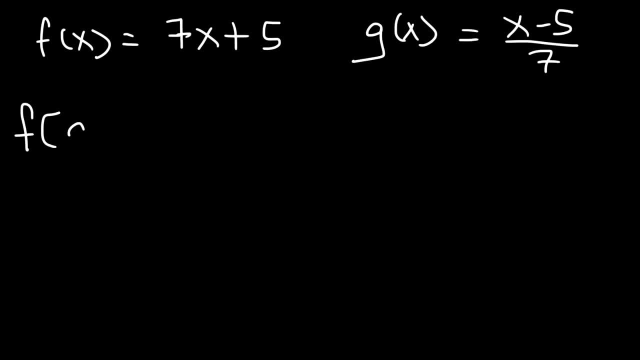 inverses of each other. Well, let's start with f of g of x. So f is going to be 7 times x plus 5.. And then we're going to take g and substitute it for x, So this is going to be x minus 5 divided by 7.. So we can see that 7 divided by 7 is 1. 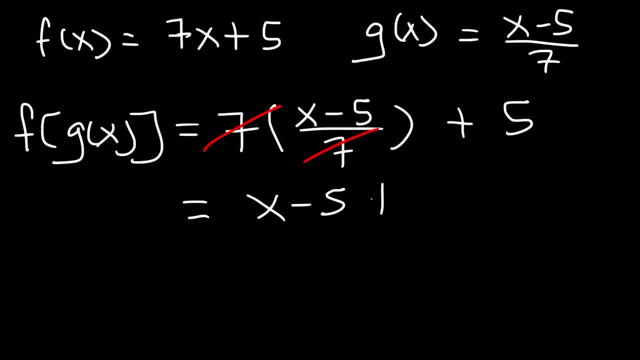 leaving behind x minus 5.. And negative 5 plus 5 adds up to 0. So we're left with x. So f of g of x is equal to x. That's a good start. Now let's see what g of f of. 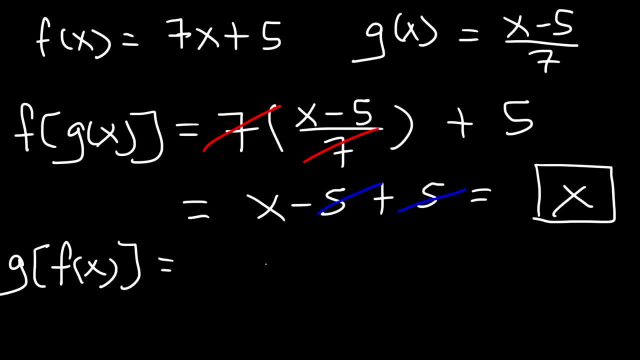 x is equal to. So let's start with the outside function g. So we have f of x minus 5 divided by 7.. Let's take f and insert it or substitute it into x, So this is going to be 7x plus 5 and then minus 5 over 7.. So 5 minus 5 is 0.. And 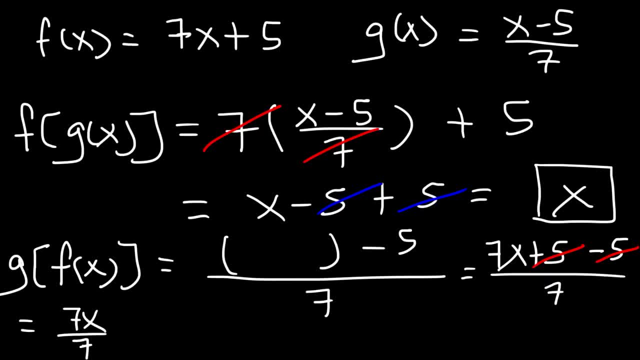 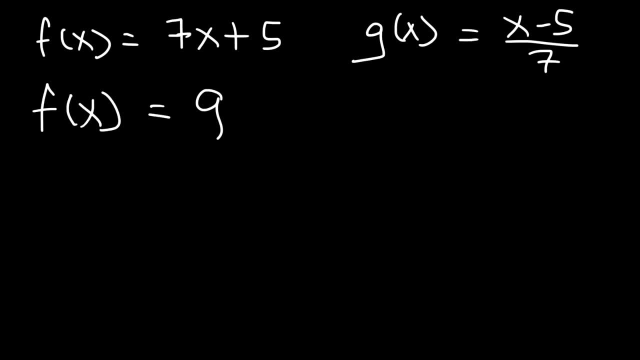 that leaves behind 7x over 7.. 7 over 7 is 1, so we get x. So therefore we can say that f and g of x are inverse. So this means that f of x is the inverse of g of x and g of x is the inverse function. 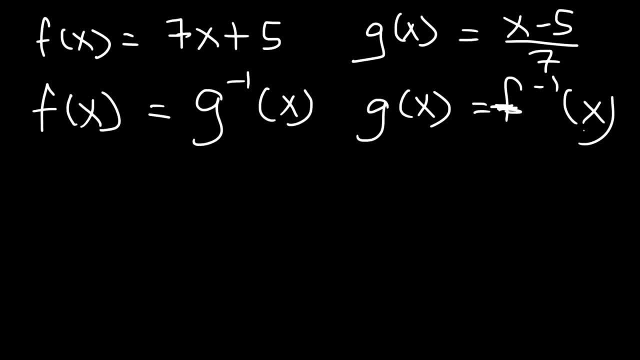 of f, of x. So let's go ahead and find the inverse of f, Just another way to verify. So let's say that y is equal to 7x plus 5.. So we need to switch x and y. If we subtract both sides by 5, we can see that x minus 5 equals 7y. And then if we divide, 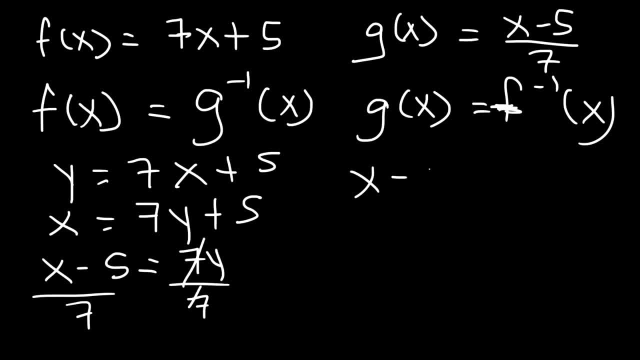 both sides by 7, we have x minus 5 over 7 is y. So x minus 5 over 7 is the inverse function of f And we can see that this is the same as g of x. So f of x and g of x are. 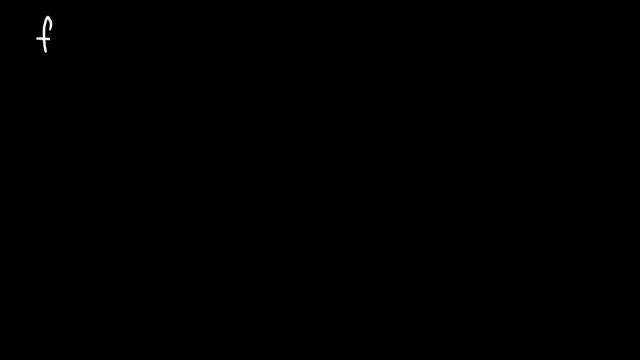 inverses of each other. Here's another problem that you could try for the sake of practice. Let's say that f of x is 5 over x plus 3 and that g of x is 5 divided by x minus 3.. So determine whether. 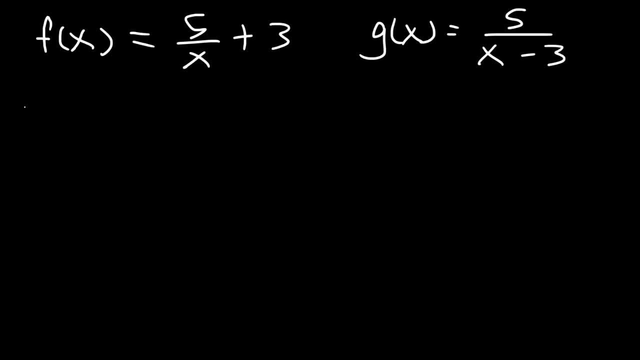 or not, if these two functions are inverses of each other. So let's start with f of g of x. So f is on the outside, So f is on the outside, So f is on the outside. And let's replace x with g of x. So I'm going to put 5 over x minus 3.. 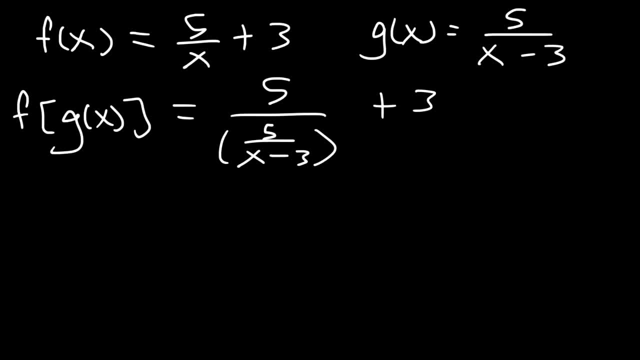 So what do we need to do here? We have like a complex fraction. What I'm going to do is multiply the top and the bottom by x minus 3.. So, on the bottom, these will cancel, And so what I'm going to get is 5 times x minus 3. 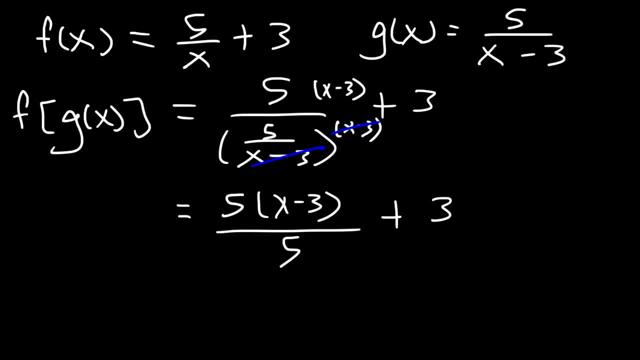 over 5.. Now notice that we can cancel 5.. So then this gives us x minus 3. And negative 3 plus 3 adds up to 0. So we get x. So that's a good start. So now let's focus on g of f of x. 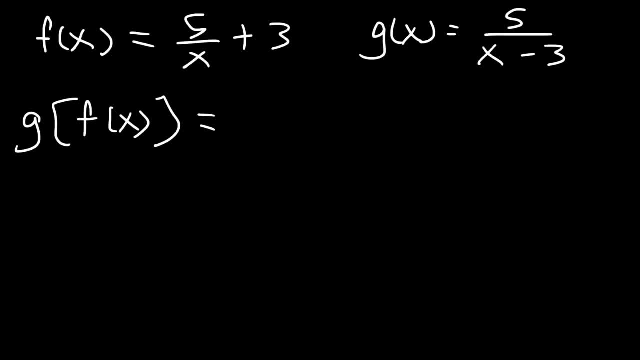 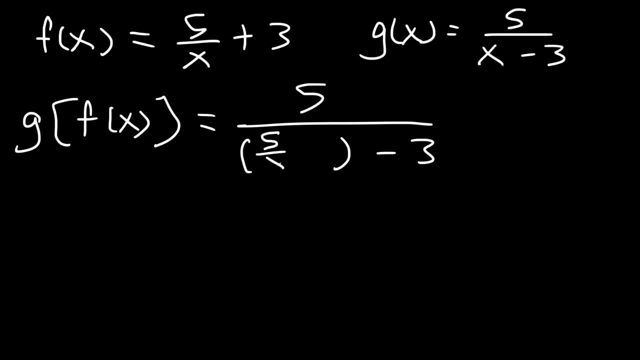 We need to put f into g, So f is 5 over x plus 3.. So we can see that the 3's will cancel, And so we're left with 5 divided by 5 over x. So I'm going to multiply the top and the bottom by x. 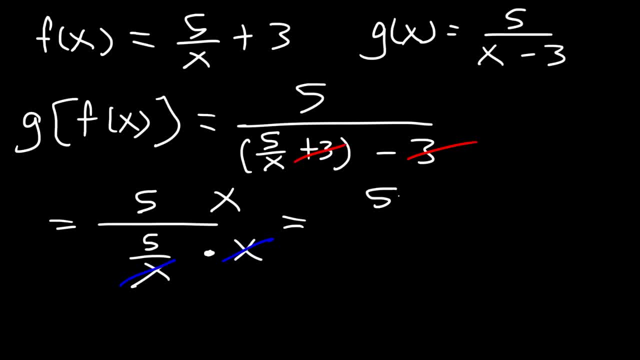 So these will cancel And this gives me 5 x over 5.. So now I can cancel 5 over x, five leaving behind x. So f of g of x is equal to x and g of f of x is equal to x. 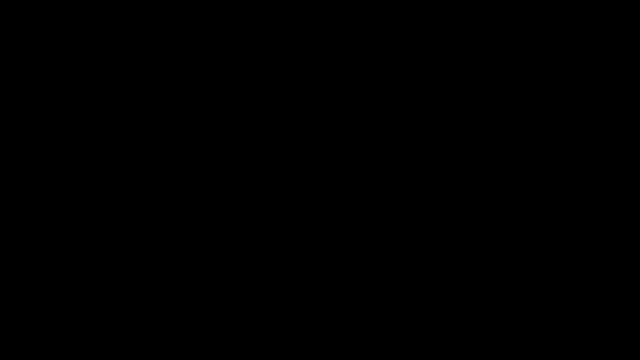 So f of x and g of x are inverses of each other. Consider this example. Let's say that f of x is 8x plus 7, and that g of x is 7 over x minus 8.. So what is f of g of x And what's g of f of x? Are these two functions inverses of each other? 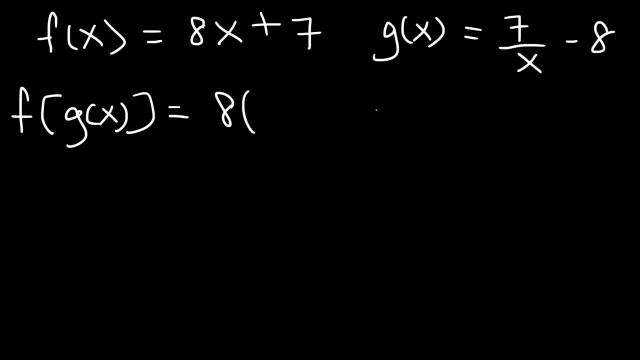 f and g. Well, f is on the outside, so let's put g inside of f. So 8 times 7 over x, 8 times 7 is 56, and then 8 times 8 is 64. Now negative 64. is equal to g of x. So f of g of x is equal to g of x. So f of g of x is equal to g of x. So f of g of x is equal to g of x. So 8 times 7 over x, 8 times 7 is 56, and then 8 times 8 is 64.. 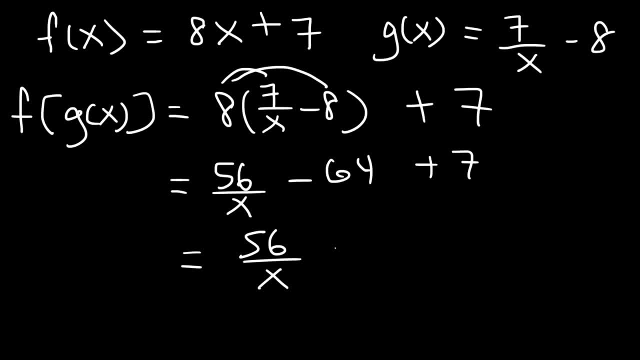 Plus 7, that's going to be negative 57. And, as you can see, this does not equal to x. So f and g are not inverses of each other. So here's the last example. Let's say that f is: 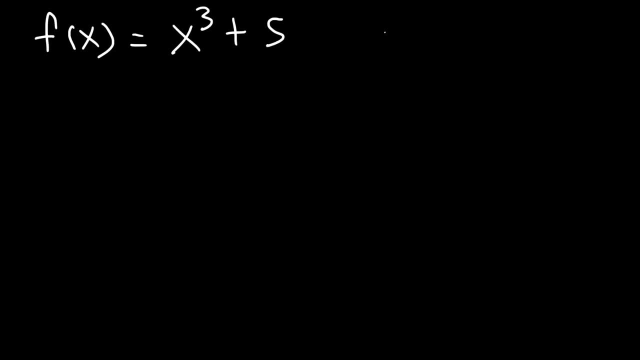 equal to x cubed plus 5, and that g of x is equal to the cube root of x minus 5.. Are they inverses of each other? No, they're not. So f of g of x is equal to g of x and that g of x is equal to. 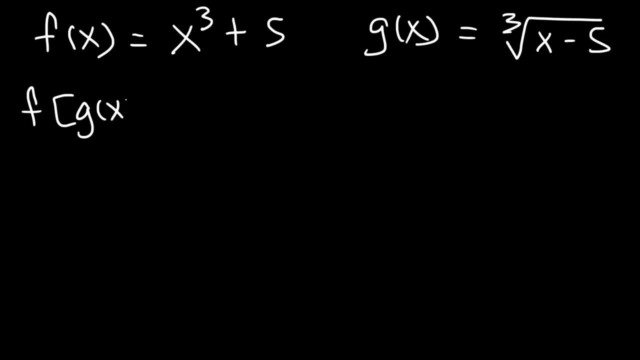 each other. Well, let's start with f of g of x, So the outside function f is x cubed plus 5.. And let's insert g into f, So let's replace x with the cube root of x minus 5..